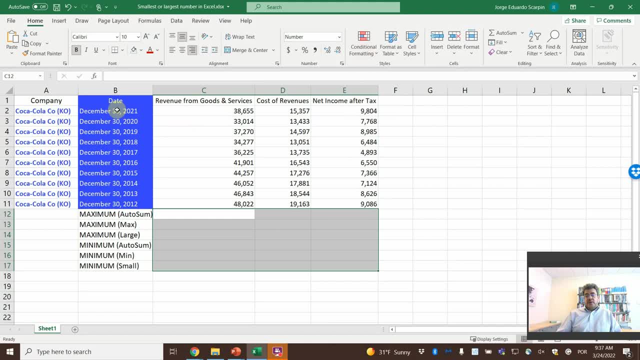 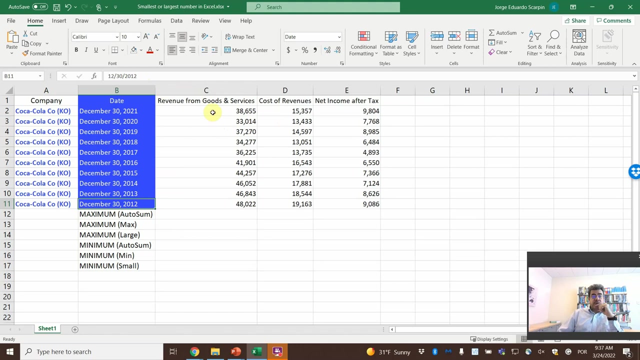 to 2021, and this is the most common in accounting or finance: Newest numbers first, oldest numbers later. So okay, largest revenue, largest cost of revenue, larger net income after tax and smallest. So the first way with the AutoSum formula select, but it works only on contiguous. 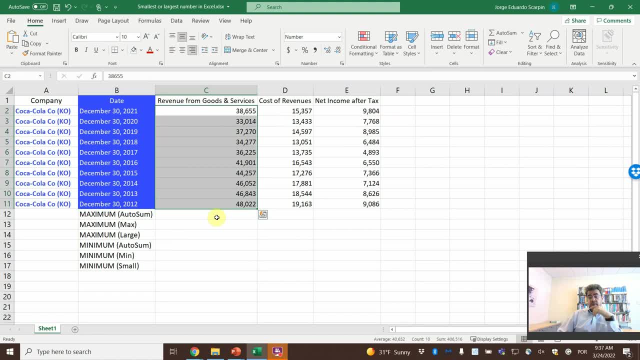 rows. The other two works with every kind of numbers: AutoSum, don't click on AutoSum. click on AutoSum. Click on the arrow here: max, it's a maximum number. Or just click here: minimum, minimum. but if you wanna go, oh, I don't want the minimum here. 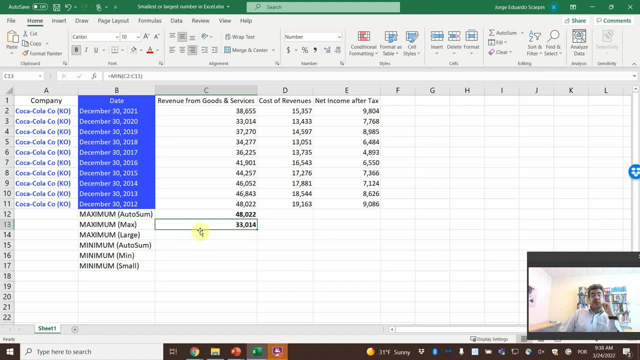 I want the minimum there. You cannot copy and paste. You need to come here, click when it's arrow and move here. If you copy and paste it will get wrong. or two functions. the first one is the max to find the largest number. max select if you want to grab. 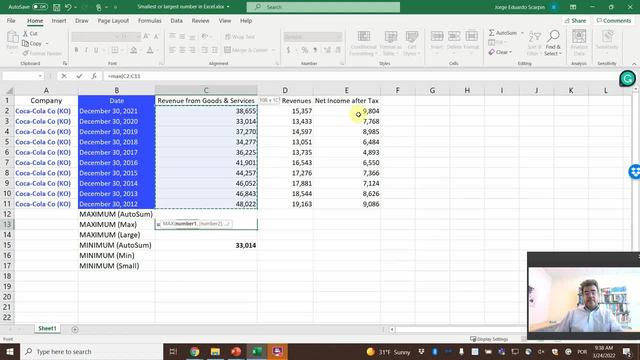 another series, for instance, revenue and net income comma the second and so on. this is what you cannot do using the auto sum. okay, but we don't want it. so, maximum number: the 48. and here, where is the 48? it is here, great. and now with the large function that is the. 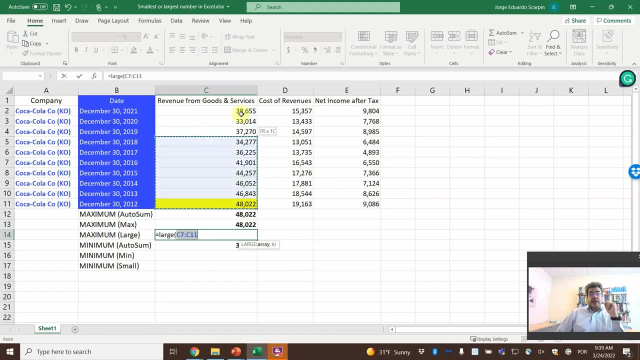 most comprehensive one, and why so? select here whoops, you can select another ones here, or comma and so on, but we don't want it, we don't, we want only revenue. you, comma, what is the k? the k is, if you want the largest number, type one, the second largest type. 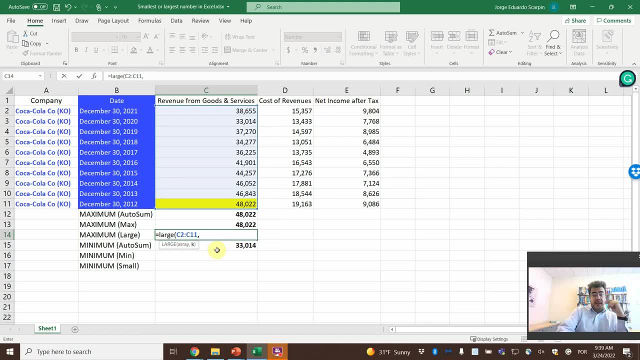 two, third, largest, type three, for instance. we want the fifth larger. it is 41, but we don't want the fifth larger, we want the largest: the same 48. and let's scope and pace here to cost of revenue and net income. so the largest cost of revenue is also 2012, where, when they got the largest, 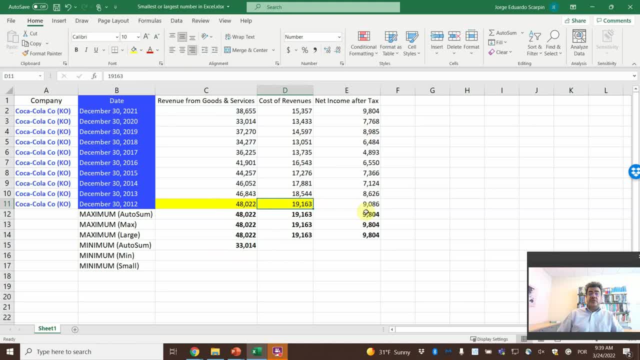 uh revenue, but the largest income is not on 2012, it is on 2021. now the minimum besides the minimum is the autosum. there is the opposite of the max formula, that is the mean formula and it works quite the same. select here if you want more numbers, comma, more numbers, and so on. the 33: 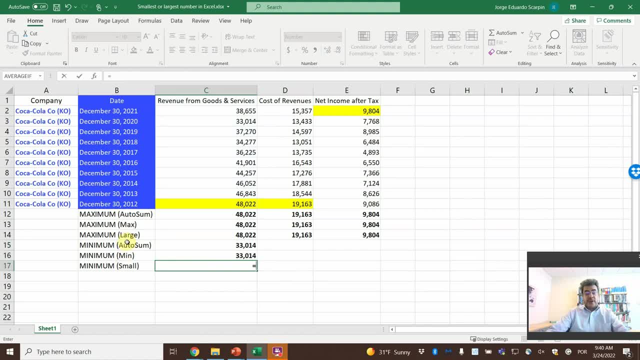 and the small function. that is the opposite of the large function. so small, select here, and then comma one. small, select here, and then comma one, small, okay, or what we want here. number one, the smallest number we can cope, and paste it to the other ones. we have them here, so let's 33, let's go on green, yellow and green. the color green reverb. 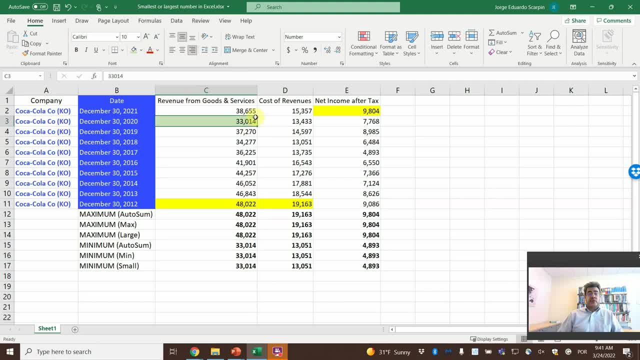 of Brazilian flags- Green- here 33.. So the smallest revenue is 2020.. Thirteen, the smallest cost of revenue is here: 2018.. And the smallest net income, 2017.. So the largest number we have- two from the same year- is smallest. three very different. 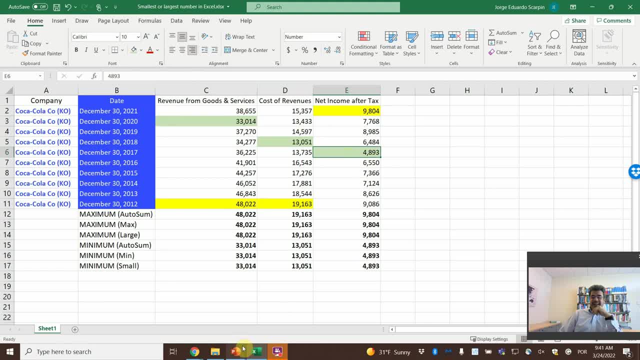 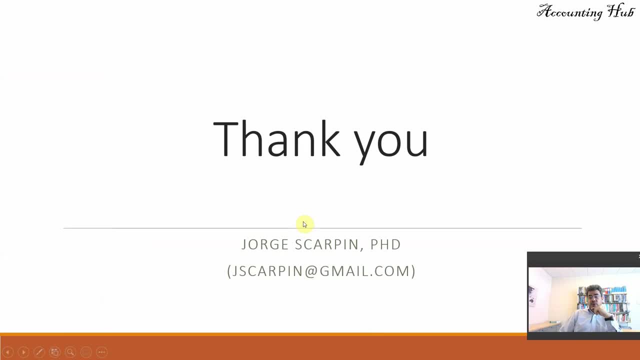 years. Easy huh. I like these formulas. They are very useful and easy to do. So, guys, thank you so much. Questions or comments? leave it here or email me at jscarpin at gmailcom. Have a very nice day and God bless you.